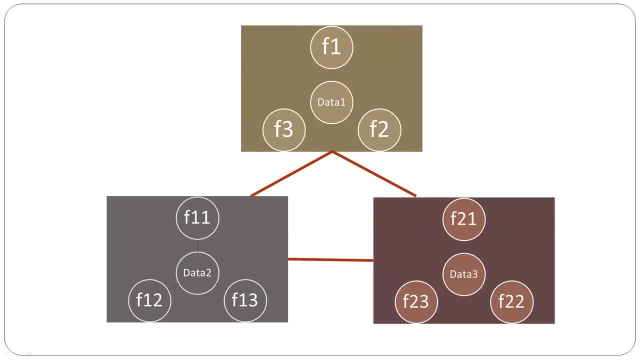 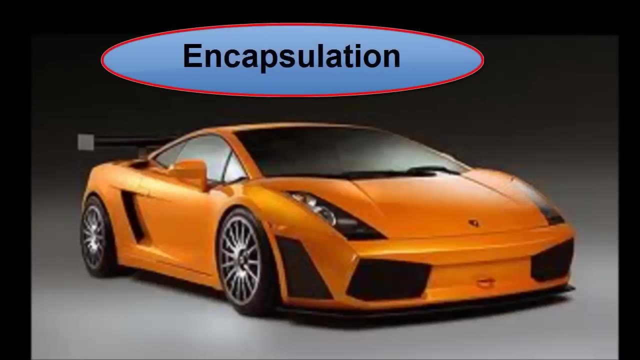 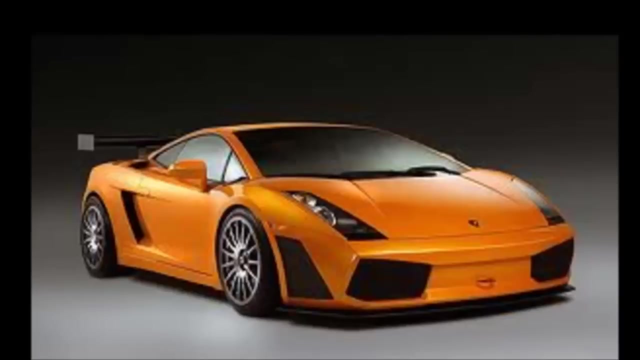 Within the object and other classes are not allowed to access the data directly. Let's discuss the object-oriented concepts: encapsulation, polymorphism and inheritance. First one is encapsulation. It hides the internal state of one object from others. It conceals the details. 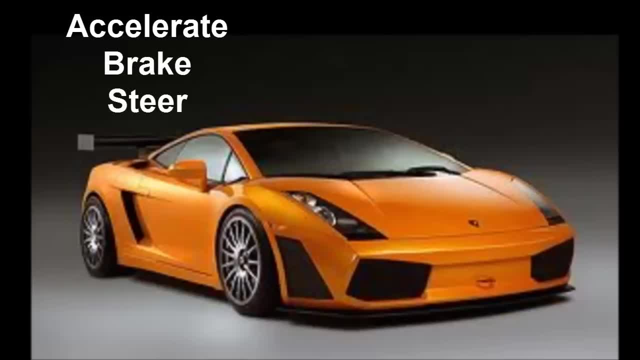 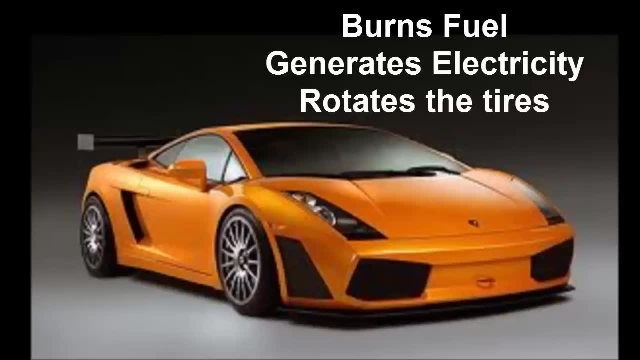 For example, to drive a car, we need to know how to accelerate, brake and shift the wheel. The car does not have to tell us about how it burns the fuel, generates electricity and rotates the tires. That information is hidden from the driver when all he wants to do is to drive to a destination. 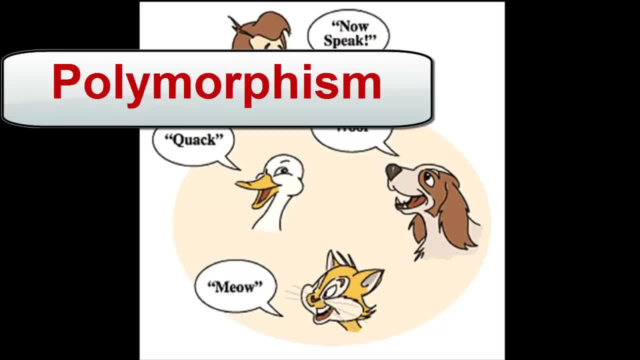 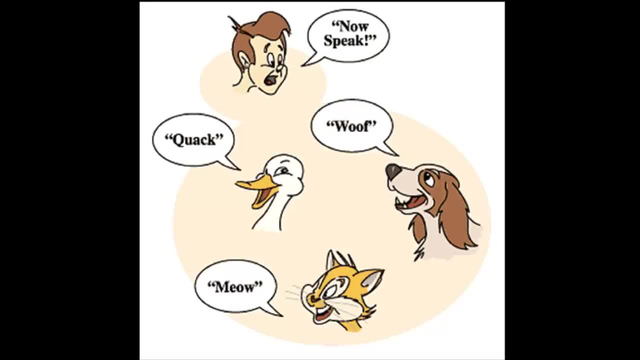 Second concept is polymorphism. It means taking many different forms. Polymorphism is the ability of one object to take many different forms. It is the ability that allows an object to be treated and used like another object. The object is not a function of a human being. 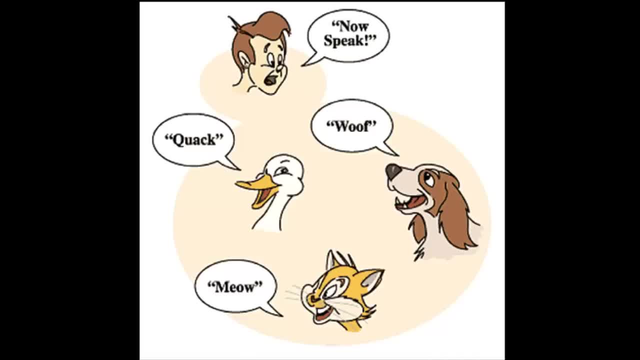 It is a part of human being. For example, we treat a duck as an animal, not just as a duck. We use a function of the object. We treat a dog and a cat also as animals. We ask them to speak. We ask each animal to speak. 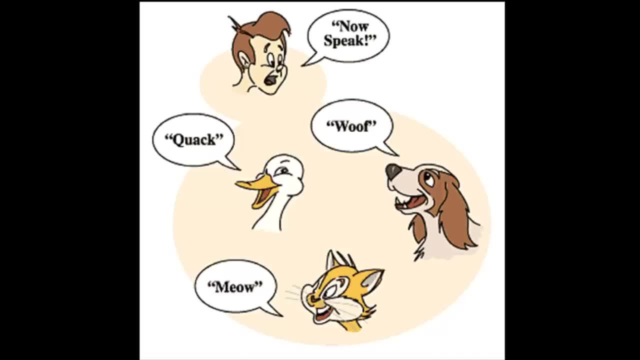 They speak in their own language. The animal speaks their language. Duck takes the form as an animal. It allows us to treat it like an animal. Polymorphism is taking the form as a form. The object is the subject and we can take it as an object. 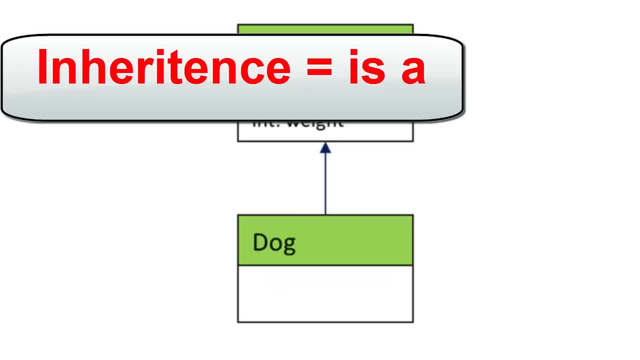 this is called, taking a different form, Inheritance. it is a relation which inherits the attributes and behaviors from their parent class. For example, dog is an animal. It means animal is a parent class and dog is the child class. The child class dog inherits the attributes like age and weight from the parent class. 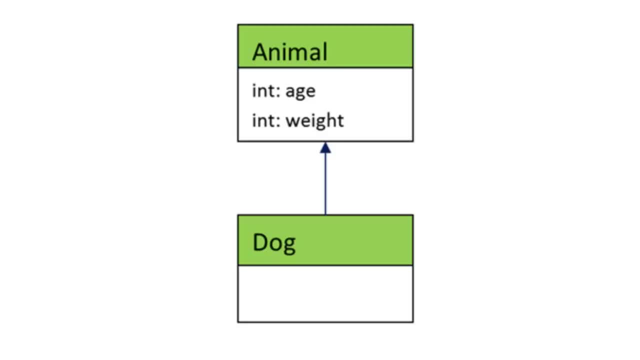 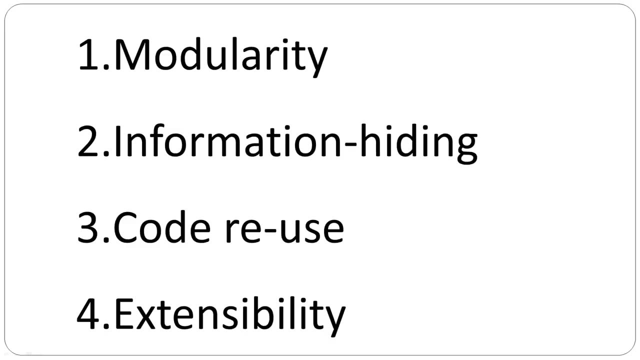 which is animal. The inheritance allows the child class to inherit the attributes and behaviors of its parent. Advantages of the object-oriented programs are: they are modular. It is easier to change one module without affecting the other. Information is hidden from other objects.